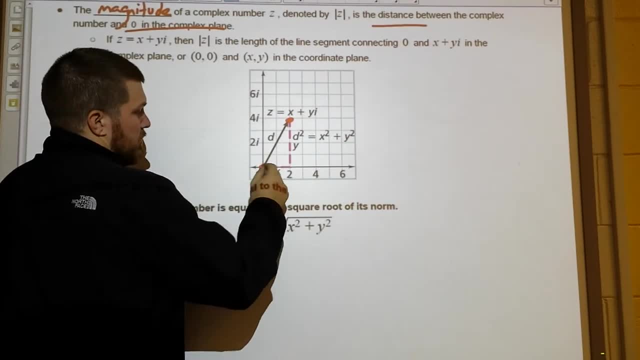 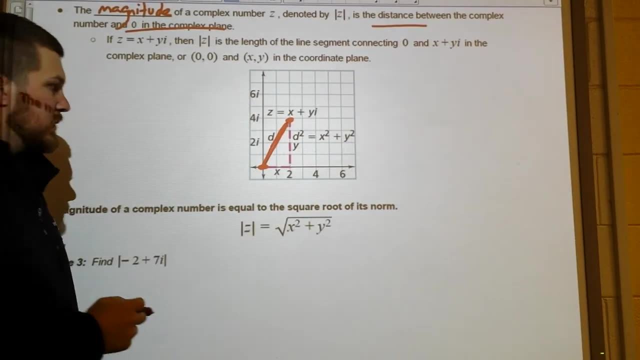 here I have a complex number. Here's my 0, 0.. The absolute value is how far away from zero this complex number lives, And I can actually figure that out using this formula. What I need to know, though, to figure it out is my. 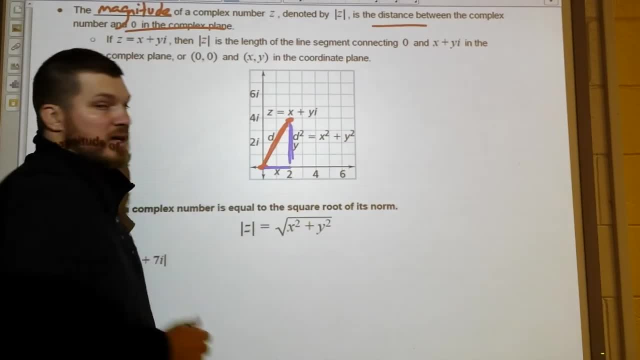 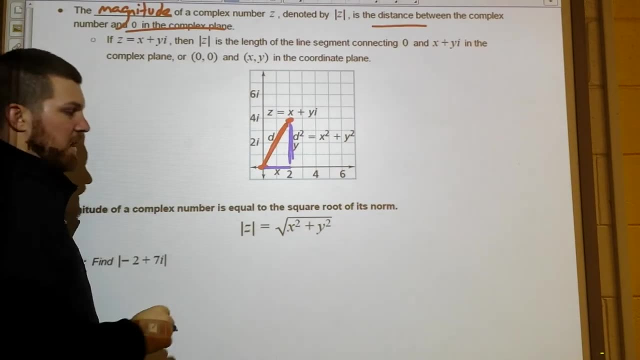 my x direction and my y direction. I just need to count those units. Once I know my x direction, I'm going to square it. Once I know my y direction, I'm going to square it, And then, to get the absolute value, I'm just going to square root. So I'm going to do this by hand And then 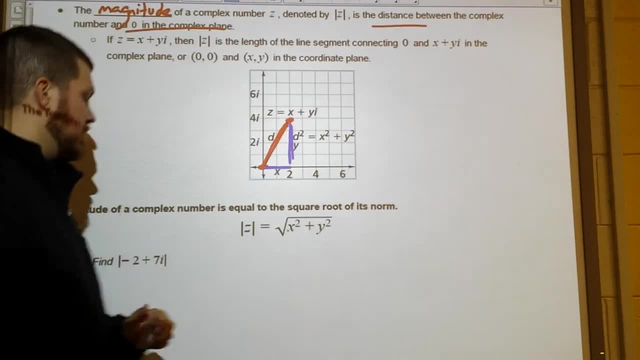 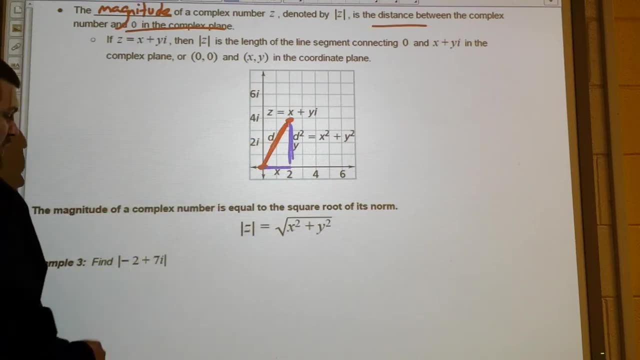 like I've done in the previous videos, I'm going to show you how to do it on a calculator. So I want to find the absolute value, on a distance away from zero, of the complex number negative 2 plus yi. Well, I know any complex number is y plus yi. 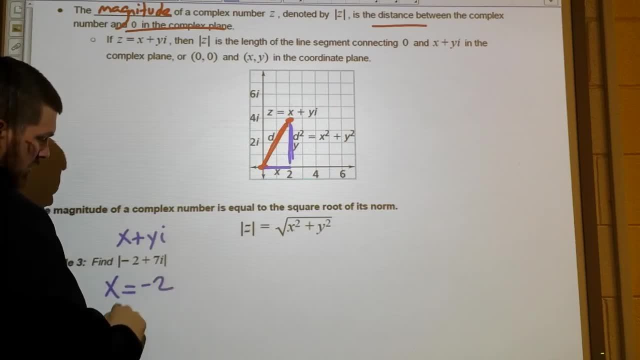 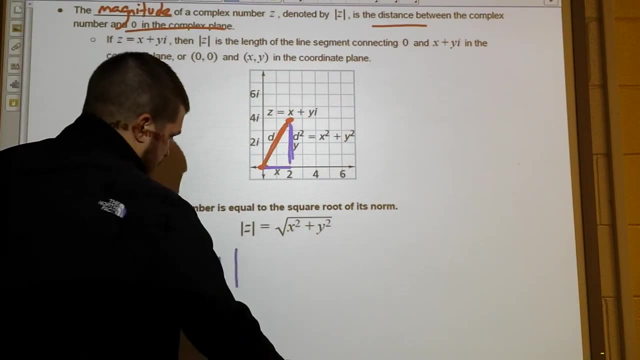 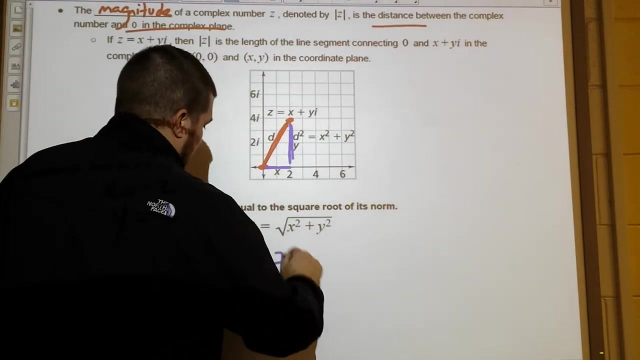 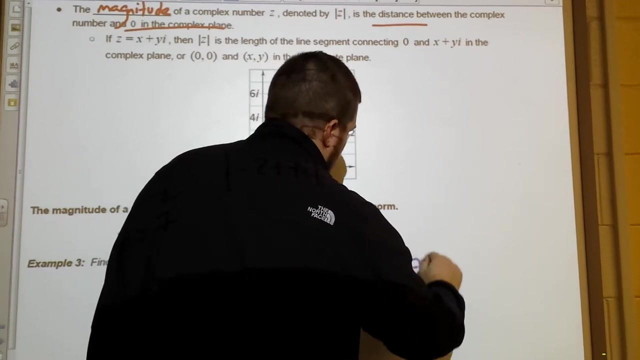 So my x is negative 2.. My y is 7.. So, based on this formula here, my absolute value- and I'm just going to call this the complex number z or sorry, the absolute value of negative 2 plus 7i, it's just going to be equal to negative 2 squared plus 7 squared. And then I want to square. 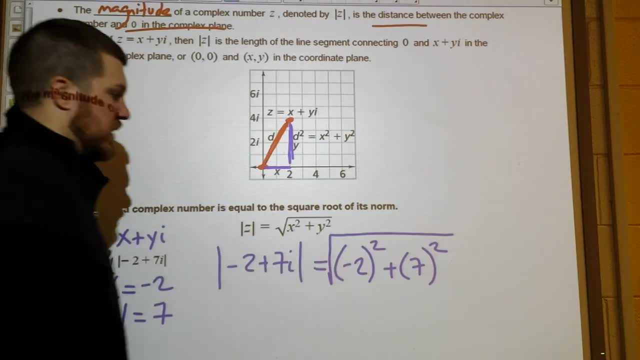 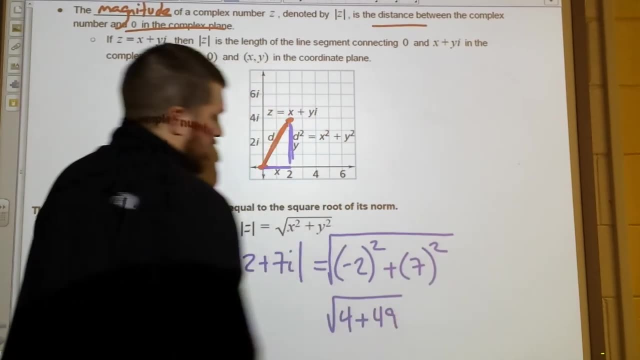 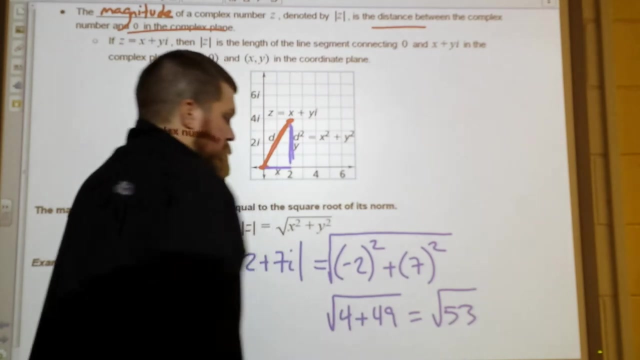 root it. Okay, Negative 2 squared is 4.. So I have the square root of 4 plus 49.. Okay, 4 plus 49 is 53.. So my absolute value is the square root of 53.. Square root of 53 doesn't work out very nice, so I'm. 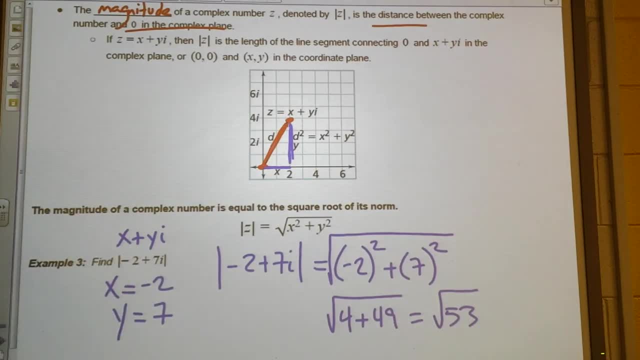 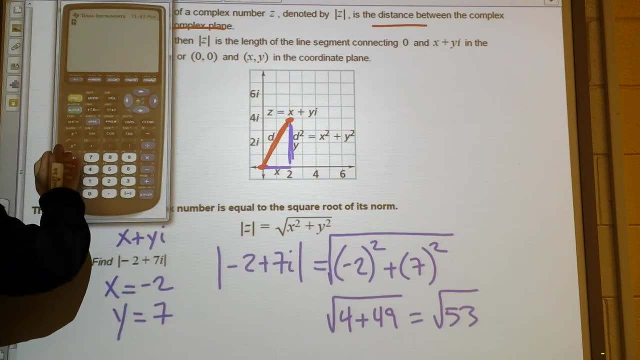 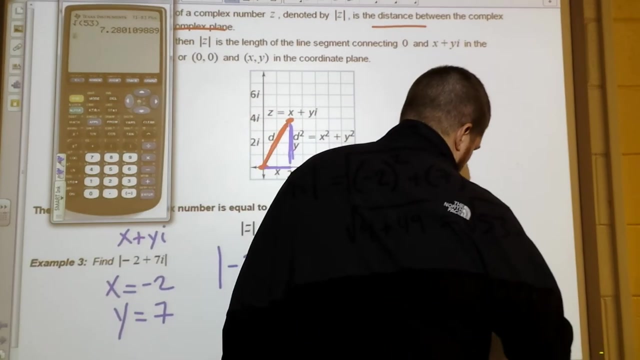 just going to leave that alone. But now I want to do the exact same problem in my calculator. First of all, let's turn square root of 53 into a decimal, because that's going to come into play in just a minute. 53 is 7.28.. Go ahead and write that down. Now. what I'm going to do is use my calculator. 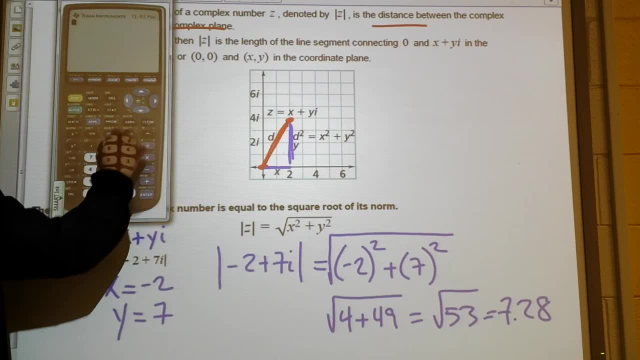 and find this exact same absolute value. First, since I see an I, I need to check my mode. make sure A plus B I is highlighted, Mine is, Make sure yours is too. I want to go to math, Go back to the complex menu CPX, and this time I want the absolute value option.